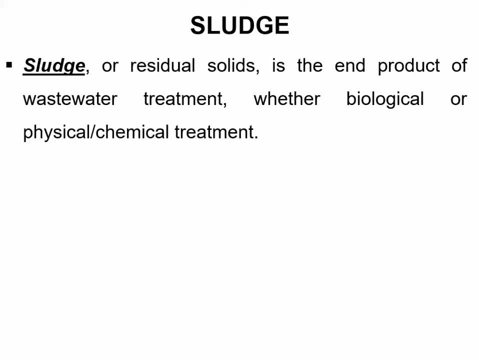 So, as we have discussed earlier that the purpose of primary sedimentation tank is to remove the suspended solids present in raw wastewater, which are mixture of organic as well as inorganic. Mostly they are organic. Similarly, in the secondary sedimentation tank, the solids which are produced in the aeration tank or trickling filter or aerated lagoon means any secondary biological treatment process. 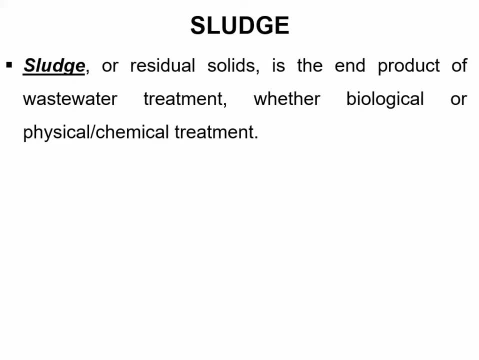 Produces the solids in the form of biomass. They are removed in secondary sedimentation tank. So both of these sedimentation tanks produce large amounts of suspended solids which contain a lot of moisture inside. Therefore, the terminology used is sludge. A sludge from municipal treatment plants is likely to contain microorganisms which may contribute to transmission of disease. 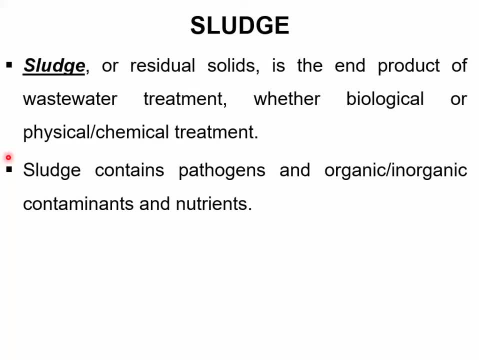 As well as organic and inorganic contaminants which may be toxic to humans or have severe effects on environment in general. For these reasons, proper handling and management of this material, this sludge, is very important component of the design and operation of a wastewater treatment plant. 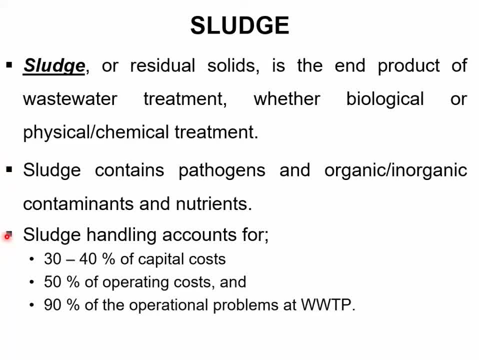 Another very interesting fact about sludge handling is That it accounts for at least 40% of the capital cost of treatment plants. 50% of the operating cost and around 90% of the operating problems are related to sludge handling and sludge treatment. 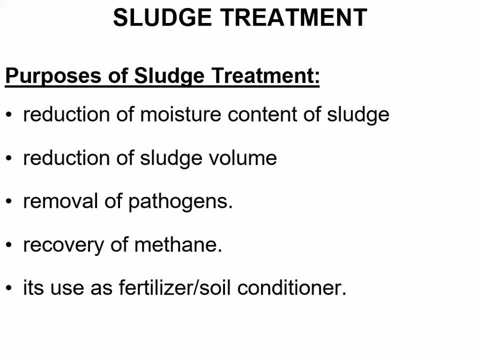 So the key objectives of the sludge treatment includes, Firstly, the reduction of the moisture content in the sludge, Thereby reducing the sludge volume. So principal objective is basically reducing the volume of the sludge And that is achieved by reducing the moisture content of the sludge. 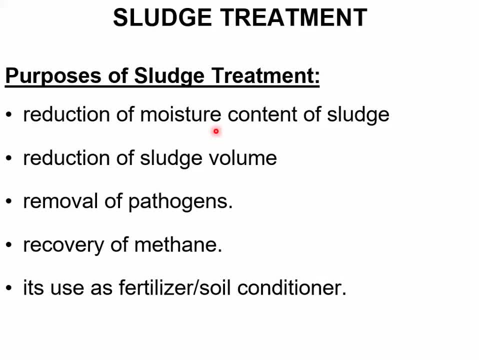 The reduction in moisture content of around 1-2% can lead to significant reduction in the sludge volume. Removal of pathogens is another objective: Recovery of methane in case of enrollment. In case of anaerobic sludge treatment, methane can be generated and recovered as a renewable energy source. 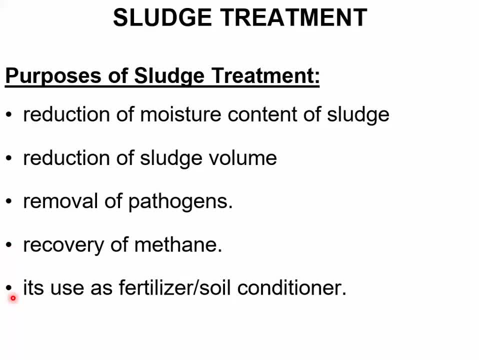 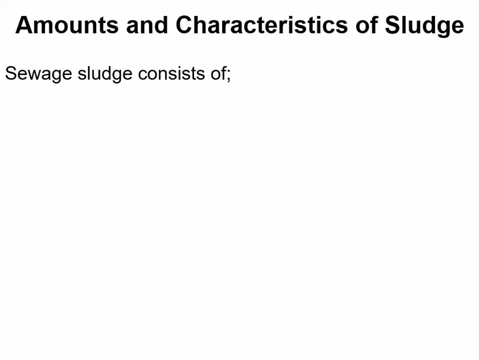 And the final objective is, if we want to use the sludge- treated sludge- as fertilizer or soil conditioner, We obviously have to treat it first. then it may be used as fertilizer. CIVIC sludge generally consists of the organic and inorganic solids present in raw wastewater. 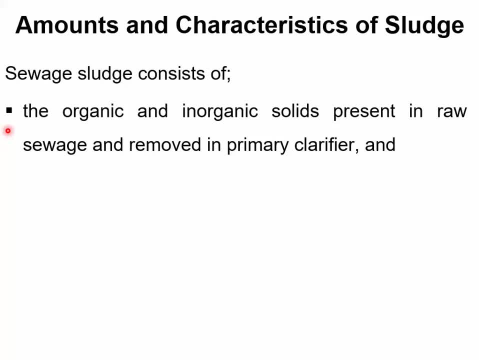 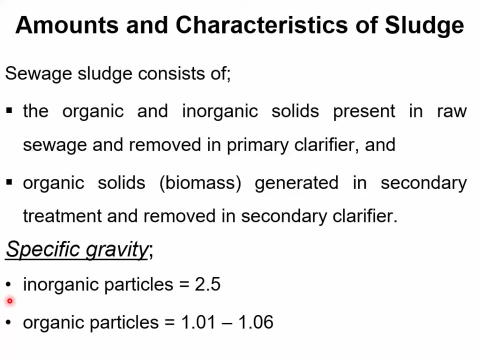 And removed in the primary clarifier. Plus the organic solids or biomass which is generated in the secondary treatment and removed in secondary clarifier, The inorganic fraction of the sludge May be assumed to have a specific gravity of about 2.5.. 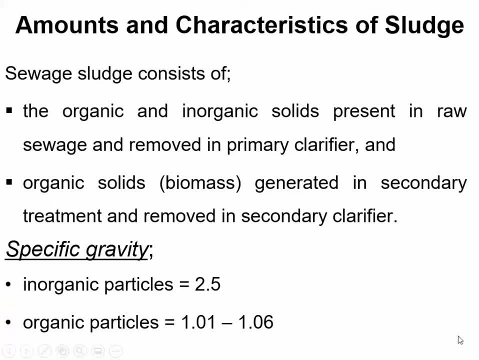 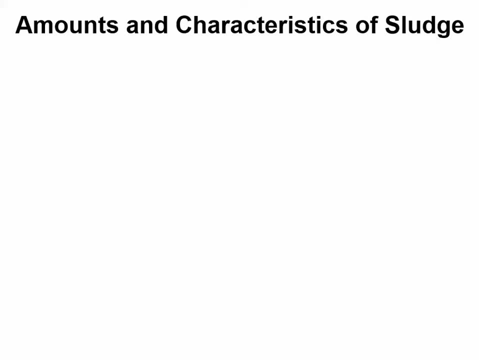 While the organic matter has a specific gravity of 1.01 to 1.06 depending upon its source and its characteristics, The domestic wastewater typically contains 100 to 350 mg per liter of suspended solids, Depending upon the flow. Communities which contain major industries may vary from this value. 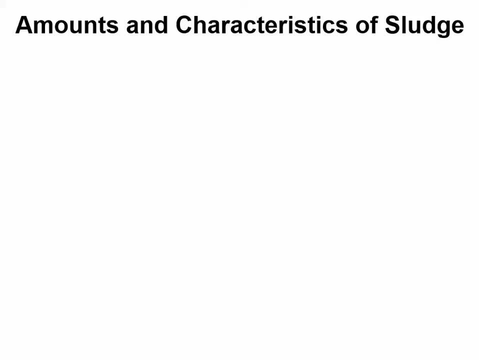 These typical values are called domestic wastewater only. Out of this quantity or concentration of solids in raw wastewater, Approximately 60% may be expected to be removed in primary clarification. The remaining portion of suspended solids goes to the secondary treatment, Where it is either oxidized. 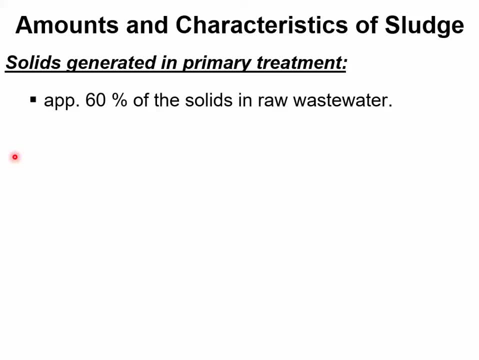 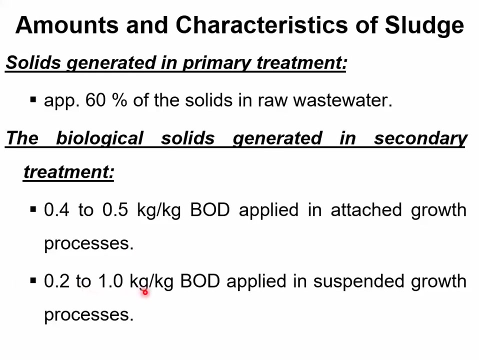 In biological treatment or it is converted into biological mass. The biological solids generated in secondary treatment May be 0.4 to 0.5 kg per kg of BOD, applied In attached process like trickling filter, Where as 0.2 to 1 kg per kg of BOD applied. 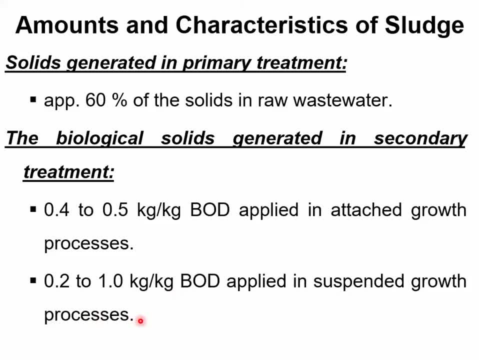 In the suspended growth processes. These are the typical quantities of solids In the form of biomass That is expected to be generated in secondary treatment. What happens in secondary treatment? The bacteria oxidize the dissolved portion of organic matter And convert it into stable end products. 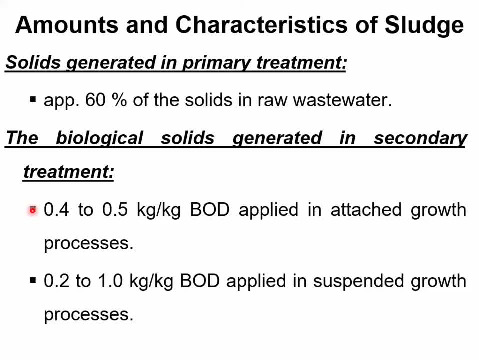 Oxidized products like carbon dioxide, And major portion goes to the biomass itself, So that biomass growth or production Is in this range for task growth process And in this range for suspended growth process, Like irrated legumes and activated sludge process. 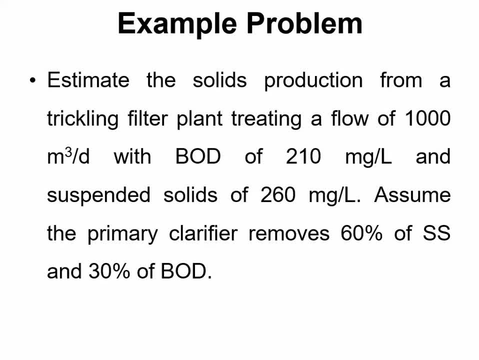 So let's solve an example problem To illustrate how to calculate the amount of solids or amount of sludge Produced From a primary or secondary clarifier. So the problem states that You have to estimate the solids production, Which means dry solids. 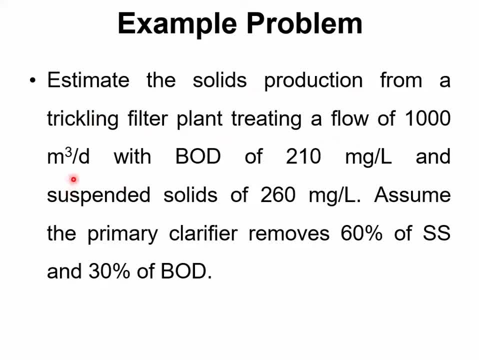 From a trickling filter plant Treating a flow of 1000 cubic meters per day, With BOD of 210 mg per liter And suspended solids concentration of 260 mg per liter. Assume the primary clarifier removes 60% of suspended solids. 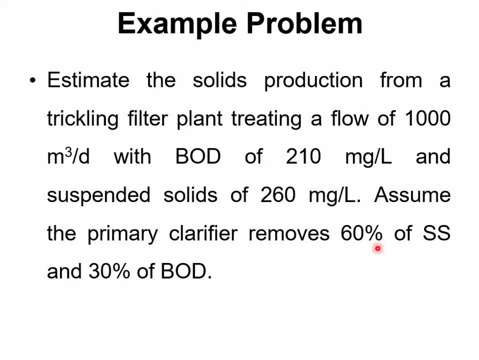 This is a typical removal of Primary clarifier And it also removes 30% of the BOD, Which obviously would be in the form of suspended organic matter. So in this 60% removal of suspended solids, This BOD removal is also included. 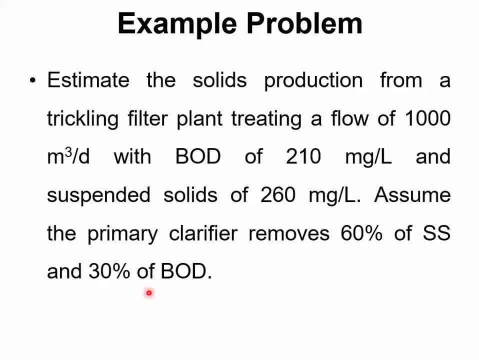 However, BOD removal is required To estimate what percentage of organic matter Went to the secondary clarifier And what was the amount of solids produced In secondary treatment And removed in secondary clarifier. So let's solve this problem For solution. first, we have to estimate. 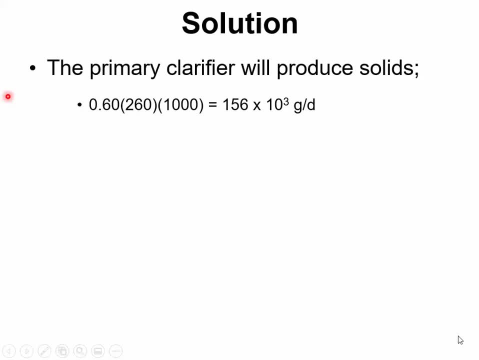 What the primary clarifier will produce as solids. So, as we have discussed earlier And given in the problem statement as well, that 60% of the suspended solids will be removed in primary clarifier, So the total amount of solids produced Can be estimated by multiplying. 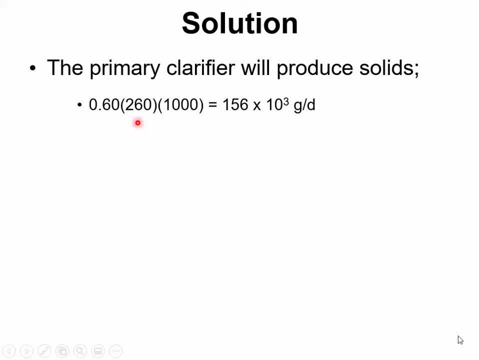 0.660%, With suspended solids, concentration of wastewater, Which is 260 mg per liter, And the total amount of discharge or flow, Which is 1000 cubic meters per day. So this is a typical calculation of loading Mass, loading of any contaminant. 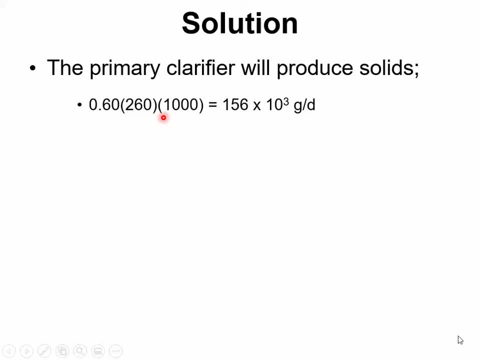 Such as we have been doing this for Calculating the mass load of BOD In various problems. So discharge multiplication, So discharge multiplied by concentration Multiplied by the fraction of The solids which have been removed in primary clarifier. So the answer is 156.. 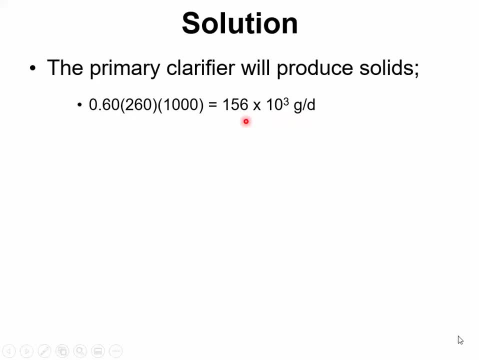 Into 10 is for 3 grams per day, Or simply 156 kilograms per day. Now, secondary clarifier Will remove the suspended solids Which are in the form of biomass And that biomass is produced In the secondary treatment processes Based on suspended and attached growth processes. 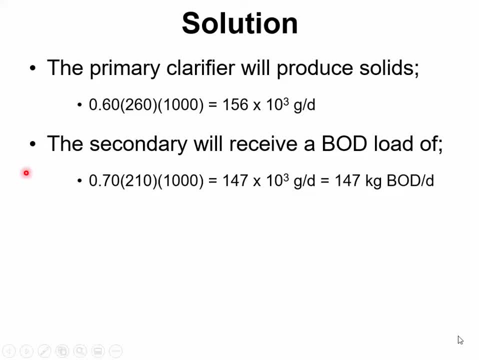 It has different value of production, But the production is linked with the Load of BOD applied to secondary treatment Which was shown to you in the previous slides. That, let's say approximately 0.5 kilograms Of biomass or solids will be produced. 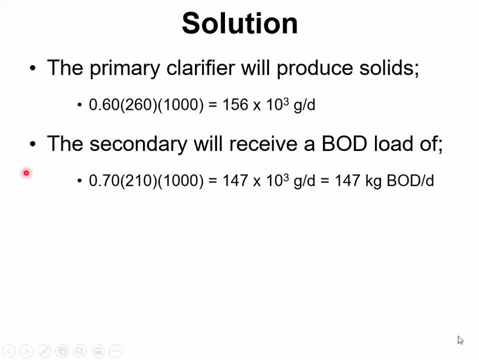 Per kilogram of BOD load Into the secondary treatment. Therefore, first we need to estimate What BOD load in kilograms Is going into the secondary treatment units. So secondary treatment will receive A BOD load of 0.7.. 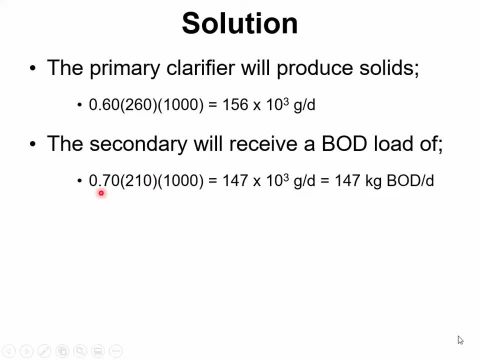 Means 70% of the original BOD concentration, Because 30% will be removed in primary clarifier, So 70% goes to secondary treatment. 0.7 of 210 multiplied by discharge Gives the value of 170 kilograms of BOD per day. 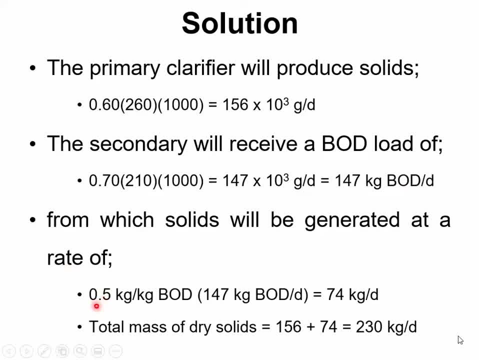 Now taking a typical value For attached growth processes From the range given on the previous slides, 0.5 kilograms per kilograms of BOD is taken here. This is the amount of solids Which will be produced as a result of BOD consumption. 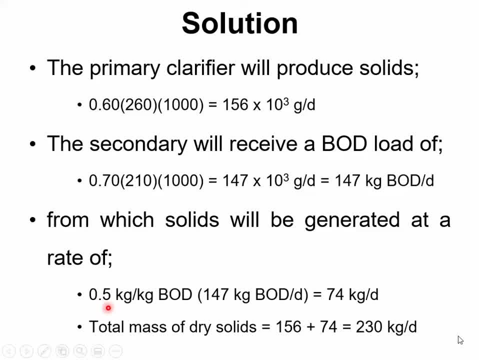 And the solids are the biomass here. So 0.5 multiplied by 147. Will give you 74 kilograms Of suspended solids, Or solids will be produced From the secondary treatment And they will be removed In the secondary clarifier. 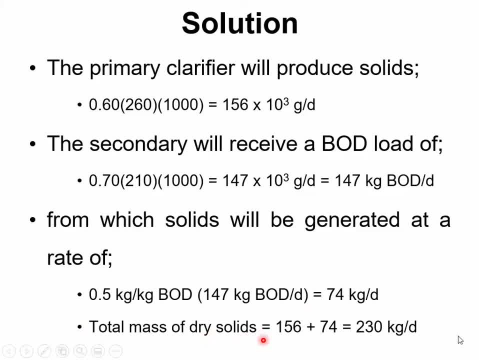 So mass of the dry solids total Which will be generated or produced From primary and secondary clarifiers will be 156 produced in primary clarifier Plus 74 produced in secondary clarifier. So a total of 230 kilograms per day. 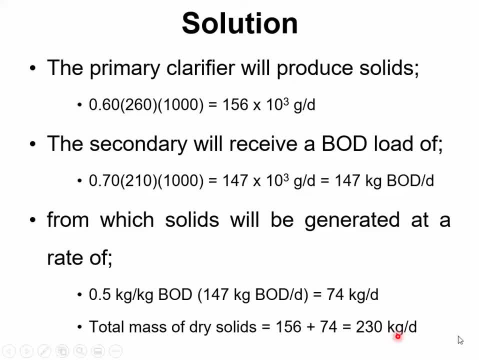 Of dry solids. Now, this Dry solids would have moisture content of, Let's say, 95,, 96% or 98%. So depending upon the moisture content, You can estimate the total mass of the sludge As well as the volume of the sludge. 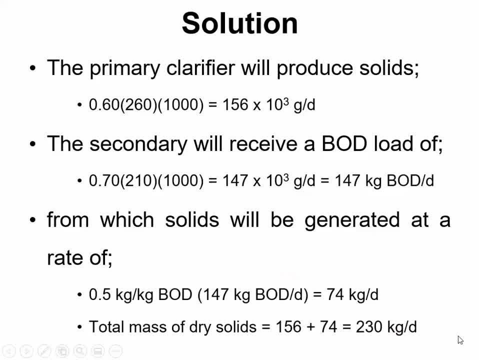 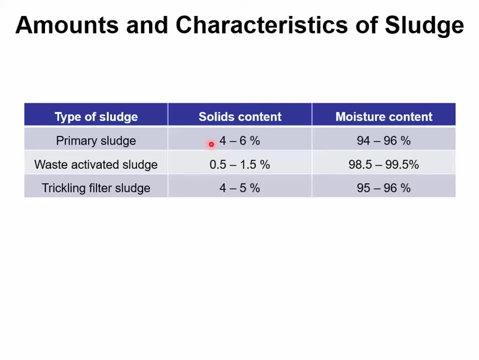 Using the specific gravity. So typical solid Contents In the primary sludge Are in the range of 4 to 6%, Whereas its moisture content Is 94 to 96%. Waste activated sludge Contains a lot of moisture content. 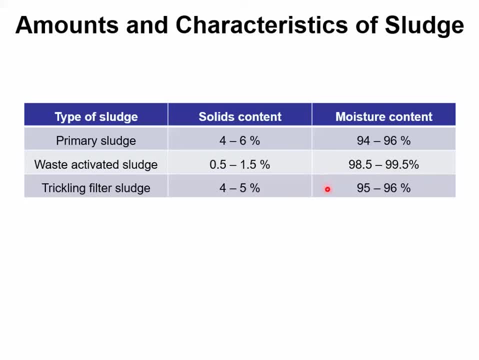 98.5 to 99.5.. Whereas trickling filter Is comparable to the primary sludge, Which contains 95 to 96% Of the moisture content And the rest are solids as 4 to 5% In the raw wastewater. 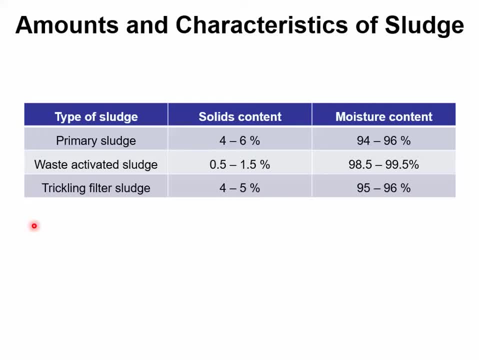 Around 0.1% In raw domestic wastewater. particularly 0.1% are solids And 99.9% is the moisture or water In the sludge. you can see In the primary and trickling filter sludge The moisture content is slightly reduced. 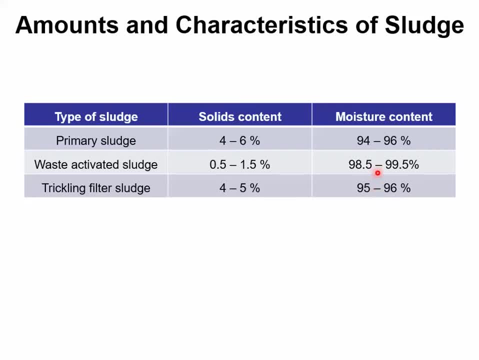 And solids contents are enhanced, Whereas in waste activated sludge This moisture content is still very high, Very close to the raw waste water, Due to this enormous moisture content Available or present in the sludge. The quantities of the sludge: 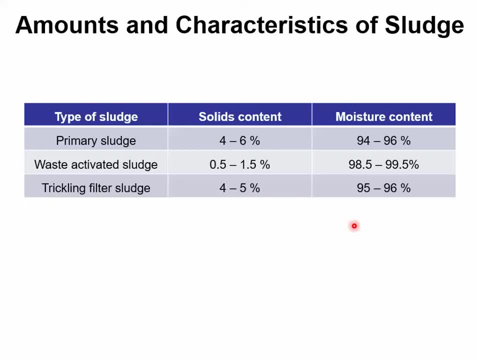 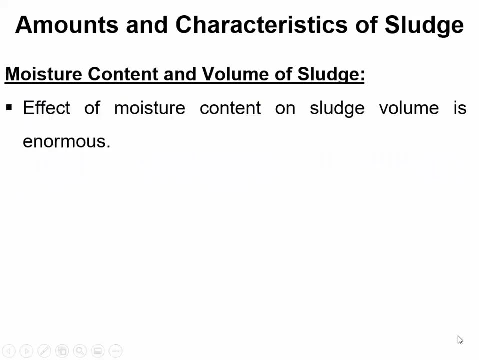 In terms of volumes Are very high. Therefore, the treatment processes For sludge Are focusing or mostly Targeting the moisture content Reduction from the sludge. The effect of moisture content On the sludge volume is enormous And sludge handling techniques. 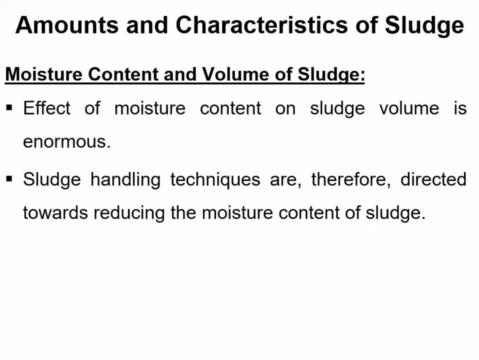 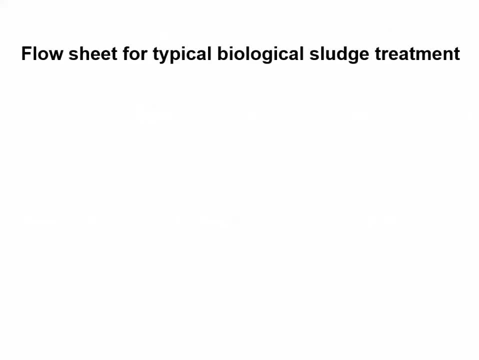 Are directed towards Reducing the moisture content And thereby Reducing the volume of the sludge, As I have mentioned On the previous slide That most of the sludge handling techniques Are directed towards Reducing the moisture content. 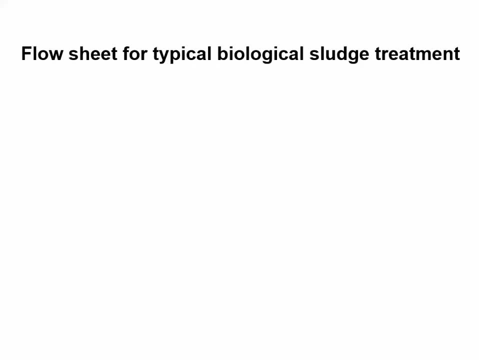 And ultimately To reduce the volume of the sludge. So a typical Flow sheet for Biological sludge treatment includes The first unit of sludge thickening. The purpose is to thicken the sludge To reduce the moisture content. 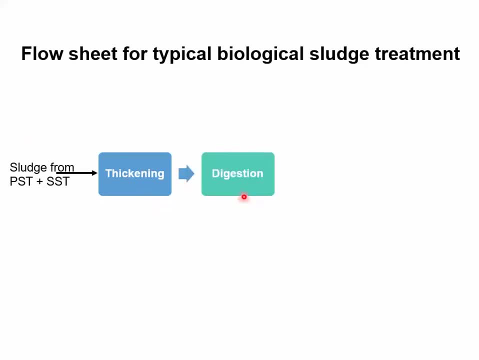 By gravity settling. Then comes the sludge digestion, Which can be aerobic or anaerobic. This is Similar to aerobic and anaerobic Digestion, or oxidation of organic matter. In this case, The organic matter Is in the form of sludge. 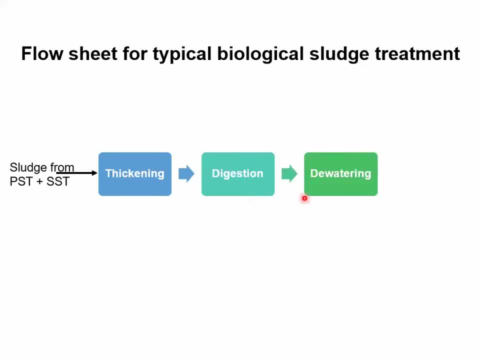 The third Unit Is the dewatering, And again The purpose of dewatering Is to reduce the moisture content. After dewatering, Dry mass of solids Are left, Which is disposed of Now supernatant. 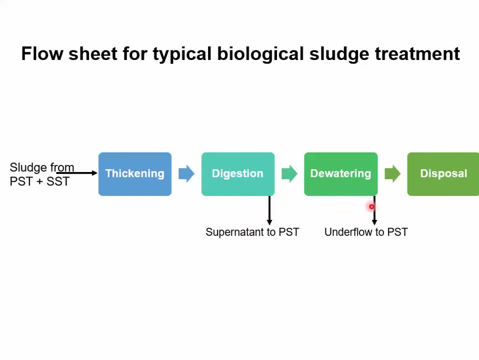 Of this digestion unit And underflow Of the dewatering unit Means the water which is Separated from the sludge In both of these units Goes to primary sedimentation tank. It is redirected back To the start of the wastewater treatment. 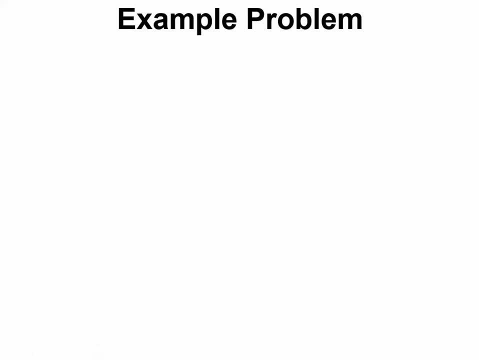 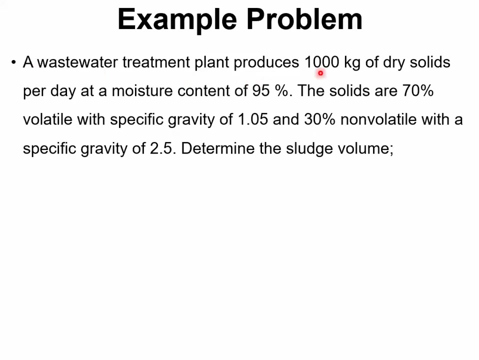 Plant. There is another example problem, Just to illustrate How the percentage moisture content Affects the sludge volume. So The waste water treatment plant Produces 1000 kg of Dry solids per day At a moisture content. 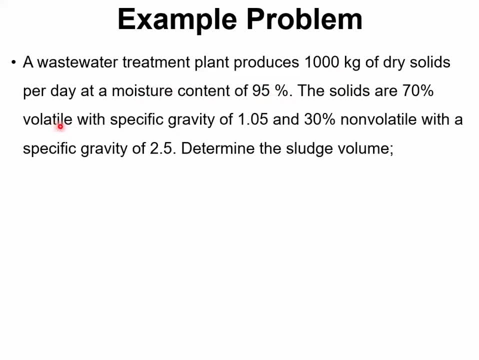 Of 95%, The solids are 70% volatile- Volatile means- organic, With specific gravity of 1.05.. And 30% are Non volatile Means, inorganic, With a specific gravity of 2.5.. We have to determine 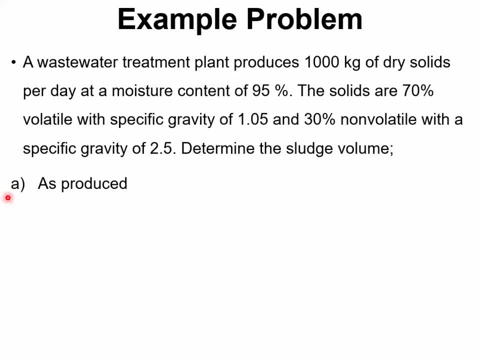 The sludge volume Has produced, And after An anaerobic digestion process Which reduces Two things. First, it reduces the volatile solids By the digestion oxidation By 50% of the original amount And It produces a sludge. 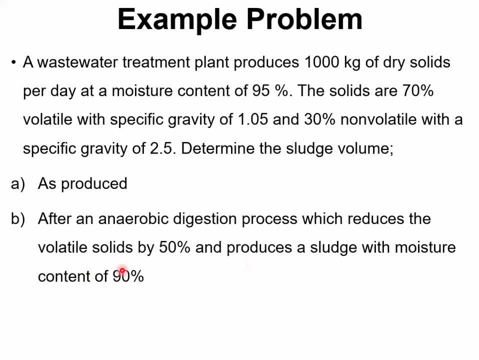 With moisture content of 95%. So it has also reduced Moisture content by a value of 5%. Originally it was 95%, After digestion it is 90%. So you have to estimate The sludge volume As produced. 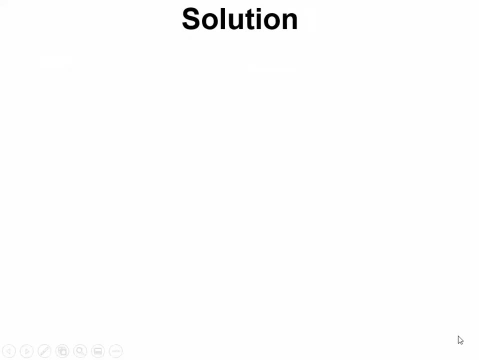 And after the digestion process. So in this situation, Let us first deal with part A. We should determine The volume of the sludge As produced. So the original mass of the sludge would be Mass of the dry solids Divided by fraction of the solids. 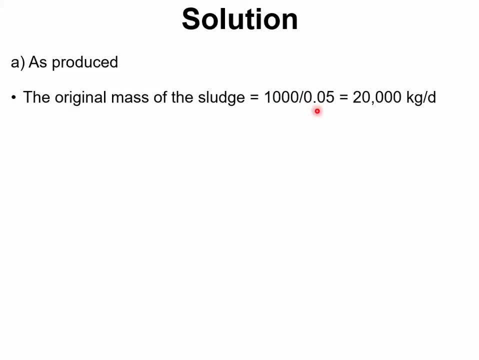 Since the moisture content Is 95%, The fraction of solids would be 0.05.. So dividing, we get 20,000 kg per day. This is the mass of sludge. Originally in the statement, Mass of dry solids was provided. 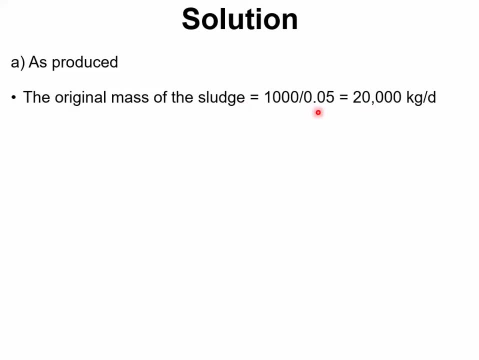 As 1000 kg. We divided it with Fraction of solids, So hence we get the Mass of total sludge, Which is 20,000 kg per day. Now, as In the statement, 1000 kg is dry solid weight. 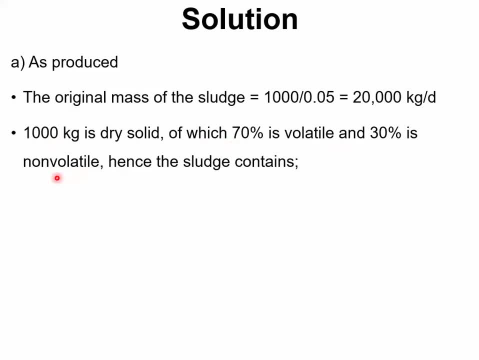 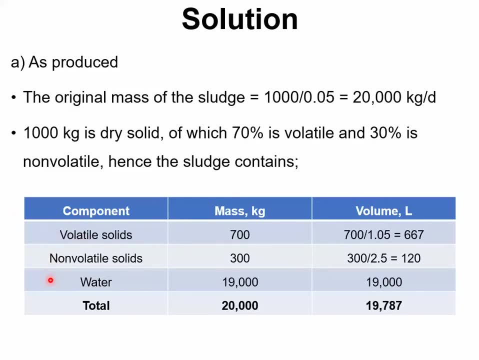 Of which 70% is volatile And 30% is non-volatile. Hence the sludge Contains volatile solids, Non-volatile solids And water as moisture. So first let us Determine the Volume of the volatile solids And then non-volatile solids. 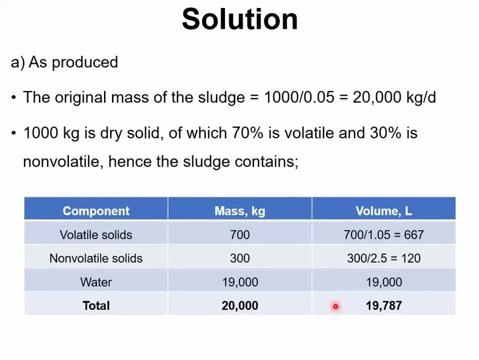 And then water And later we will sum up this. To calculate the total volume of sludge For volatile solids, The mass is 70% of the total 1000 dry solids, So it is 700 kg To get the volume. 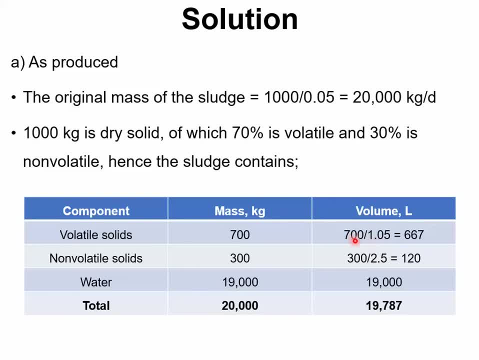 We can divide it With the specific gravity. So 700 divided by 1.05.. Gives 667 liters. Non-volatile solids Are 300.. Because they are 30% of the 1000.. So 300 kg divided by. 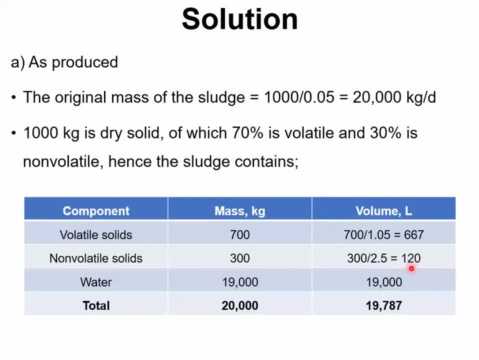 Their respective specific gravity Of 2.5. It gives the volume of 120 liters. Now what is the water? If 20000 is the total mass of sludge And 1000 is the dry solids, The mass of water would be. 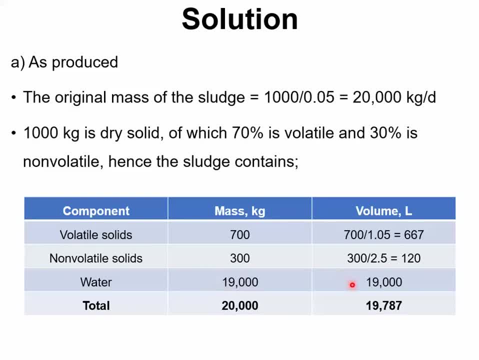 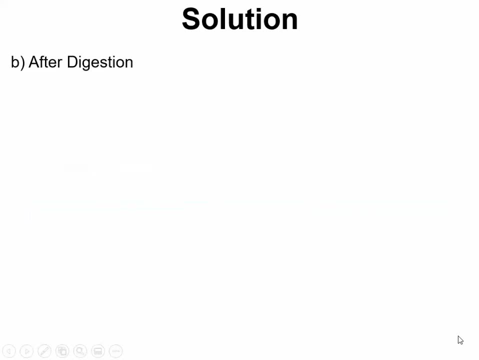 19000 kg And volume of water Would be same, Taking the specific gravity as 1.. So the total volume Of the sludge would be 19787 liters. So After digestion, Which is part 2. Of the problem, 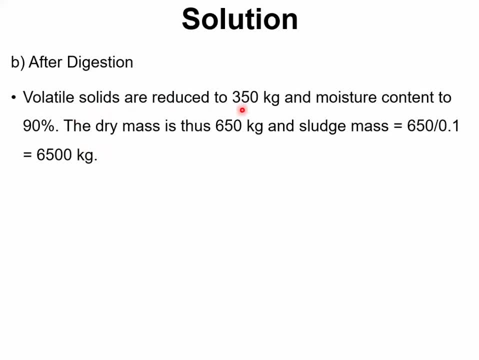 It was stated that Volatile solids are reduced To 50% of the original, So originally They were 700 kg. After 50% reduction They are left as 350 kg And moisture content Has been reduced to 90%. 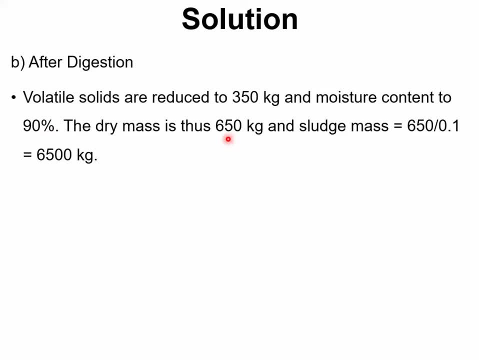 Therefore, the dry mass Will be reduced to 650 kg Because Volatile solids, Which were 300.. Remains same, Whereas Volatile solids Which were 700. Now they have been reduced to 350.. So 350 plus 300.. 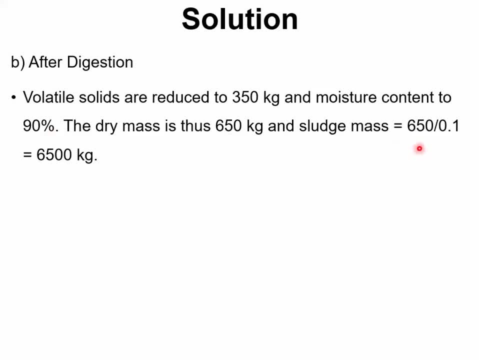 The total dry mass Would be 650 kg And the sludge mass, Using this moisture content And solids fraction of 0.1.. Dry mass of solids Would be the total mass Of the sludge As 6500 kg. 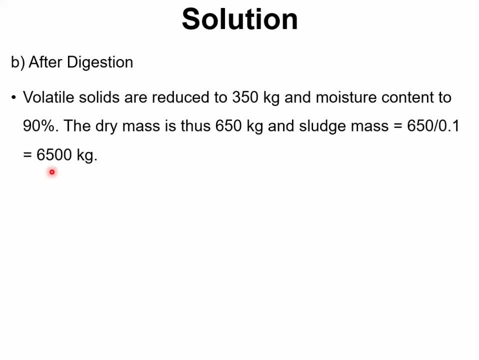 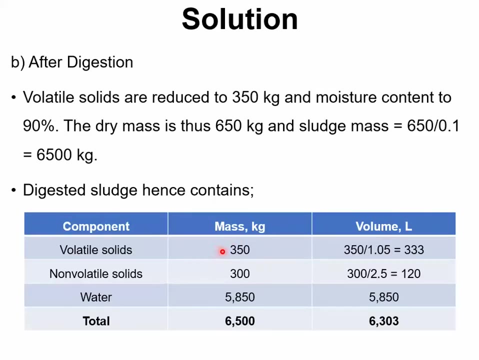 So now you can estimate, Or you can imagine, How much reduction In mass has been achieved As result of digestion process. Originally it was 20000 kg, Now it is 6500 kg, And digestive sludge Would contain these elements. 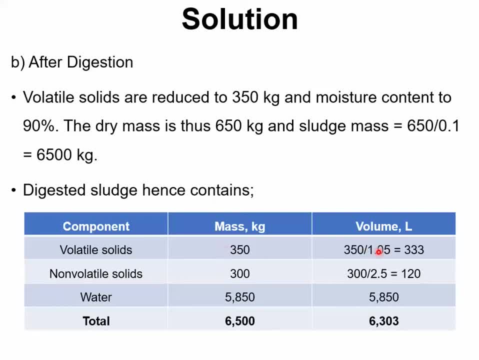 Volatile solids. Originally they were 700.. So its volume would be 333 liters. Non volatile solids, Unchanged because They are not affected by digestion, And the water now Subtracting 65.. 650 kg From 6500.. 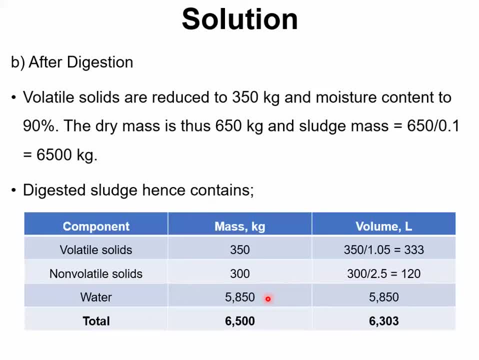 Gives the value of 5850 kg And the volume would be the same, The total volume of the sludge Would be 6303. liters. So as compared to Originally the 19887. Something, Now the volume has significantly. 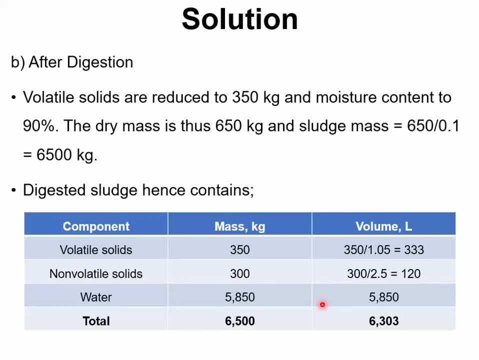 Reduced And, principally, it has been reduced Because of the moisture content. As you can see, The change in the volume Of the volatile solids Is not that significant And non volatile solids Volume is not changed. The only significant change. 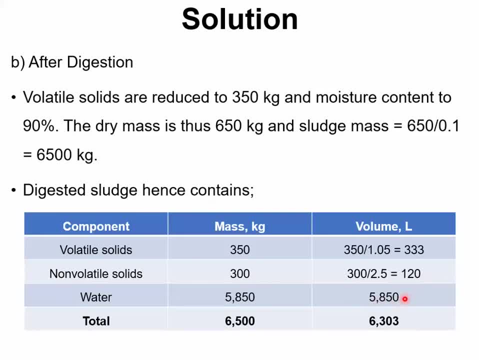 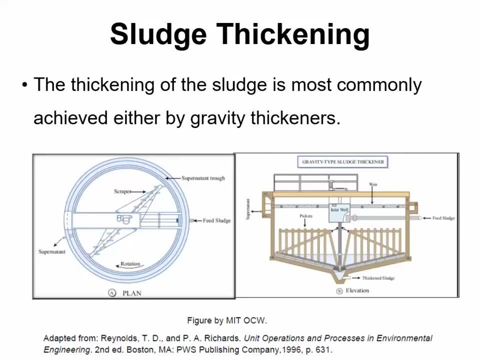 From 19000 liters To 5850 liters Is in the water Mass or water volume Because of the change in Moisture content. The first unit Applied for sludge treatment Is sludge thickening. The purpose of sludge thickening 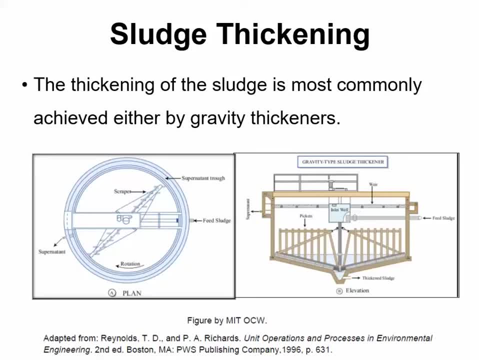 Is to reduce the moisture contents And to increase the percentage of solids In the sludge. The thickening of the sludge Is most commonly achieved By gravity thickness. The other methods used are Flotation and Centrifugation. 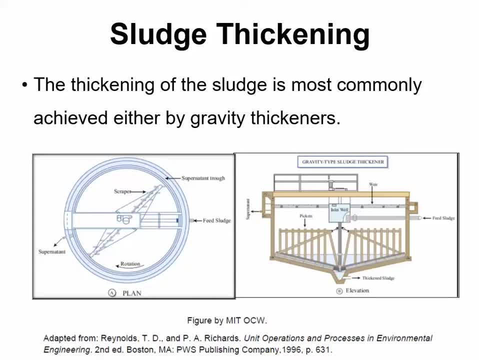 The gravity thickness Are most commonly used. They are just like sedimentation tanks. As you have studied The primary and secondary sedimentation tanks, This is also a sedimentation tank In which sludge is Applied And it settles down by 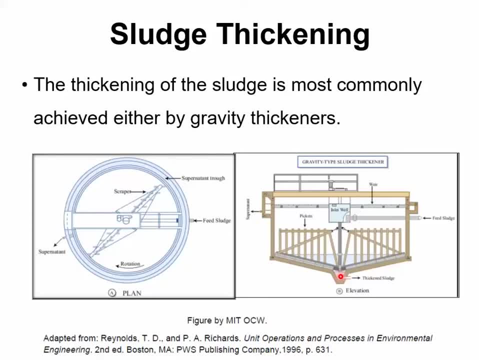 The mechanism of Type 4 settling. This is referred to as compression settling. If you recall, We discussed that in Water treatment topic of sedimentation. Sludge thickening Involves type 4.. Or compression settling In just a sedimentation tank. 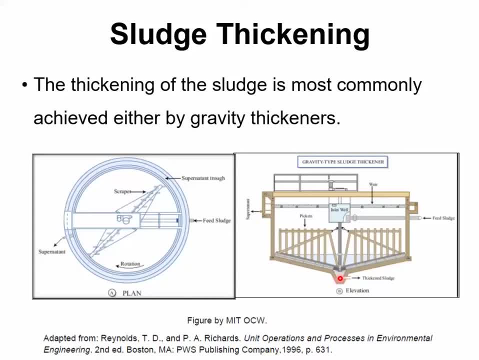 The thickened sludge Is removed from the bottom And the supernatant Which is separated from the sludge. The water Is removed from the top And returned back to Primary sedimentation tank For the treatment. The second treatment unit. 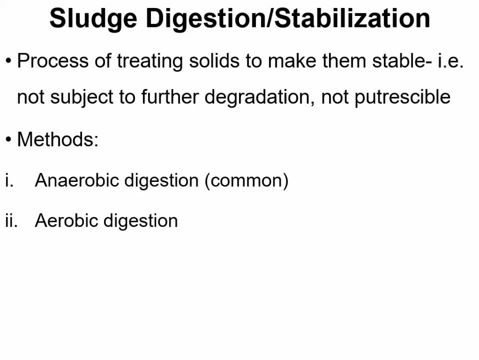 Employed for sludge treatment Is sludge digestion. This is the process of treating The organic solids To make them stable, To oxidize them, basically, To make them stable So that they are not subject To further degradation Or they are not. 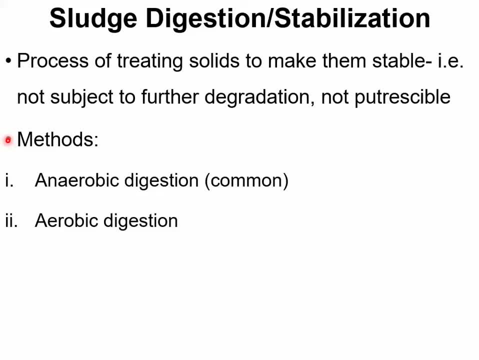 The methods employed For sludge digestion Includes anaerobic digestion. Aerobic digestion- Both of these are Biological processes. The other methods include Alkaline stabilization, Composting or incineration. Out of these methods, Anaerobic digestion. 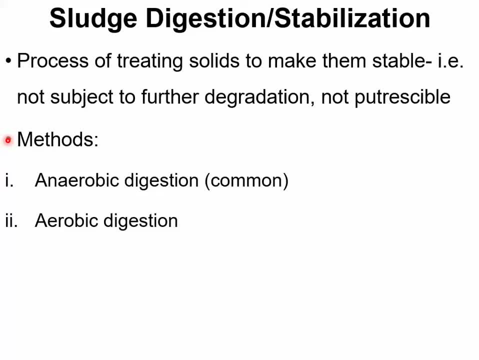 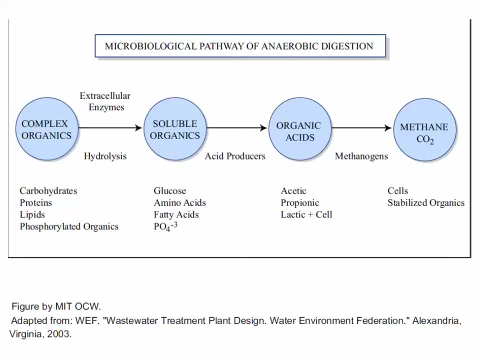 Is commonly used Because of its advantages, Such as In comparison to Aerobic process, And the other advantage Is the production of Methane as bi-product of digestion. This figure represents The overall Anaerobic digestion process. 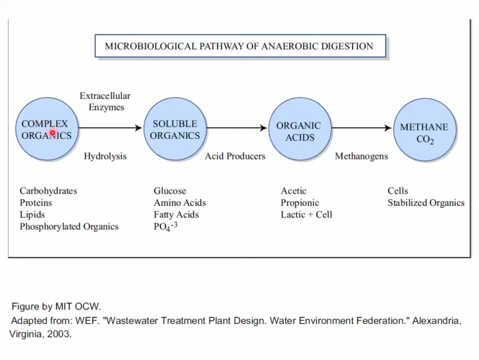 So in the first stage of The process, Complex organic compounds Such as carbohydrates, Proteins, lipids Are broken down With the help of enzymes To produce Soluble organic Or simpler organic products Such as Glucose, amino acids, fatty acids, etc. 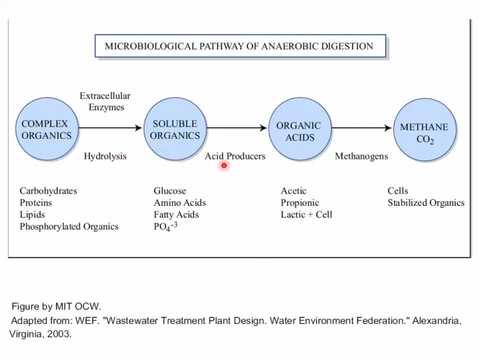 This process is known as Hydrolysis. Then Acid forming bacteria, Which are also known as Acid producers, Convert these Soluble organic products To organic acids Such as Methane forming bacteria, Which are also known as. 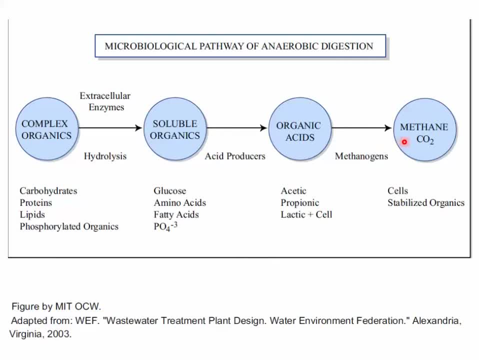 Methanogens Into methane and carbon dioxide And further cells, Obviously biomass, New bacterial cells And stabilized organics. This overall Process, Particularly The last one, Which is methane forming bacteria Which converts the organic acids Into the methane. 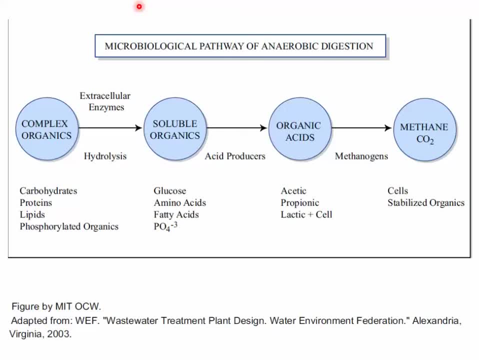 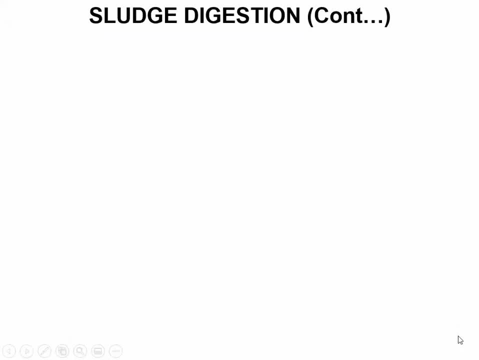 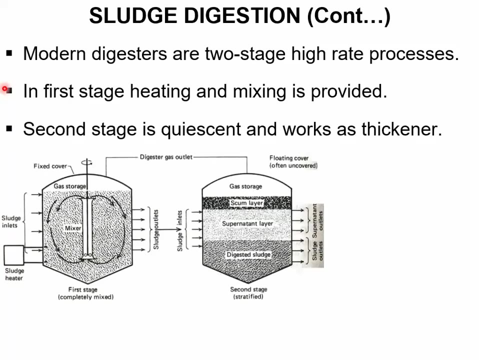 And to Reduce the pH Range of 6 to 8.. And to adjust the pH, Lime is added If required. Modern digesters are Two stage High rate processes. In the first stage, Heating and mixing is provided. 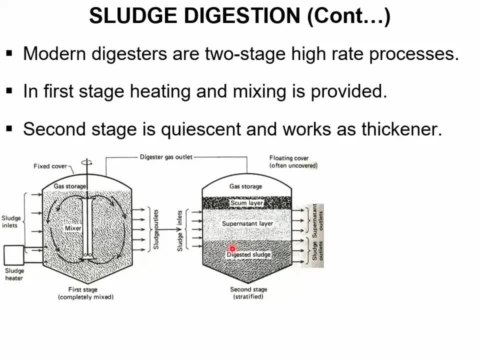 Where, as Second stage, is Quenched and works as Thickener At the bottom. This is digestive sludge, This is supernatant layer, And then scum layer And finally the gas storage Above it. Similarly here in the first stage, 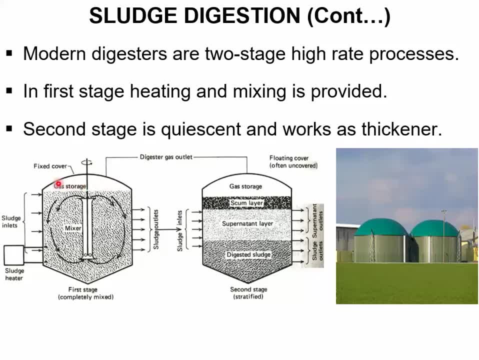 Since the reaction starts, So gas can be produced. So gas storage is provided At the top of this sludge. Now why? The sludge is heated In the first unit, So the temperature Has a significant effect On this anaerobic digestion reaction. 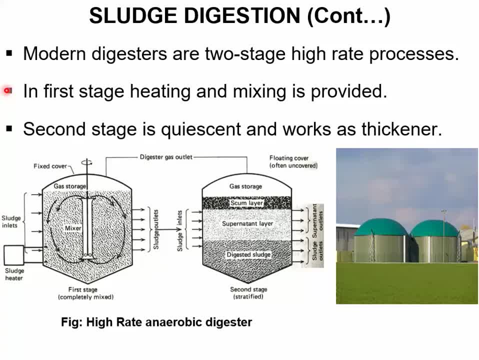 And it can significantly Reduce the required retention times, Hence the volume Of the digestive. For example, At 20 degree Celsius, If 10 days are required, 10 days of retention time. For 35 degree Celsius, Only 2 days would be required. 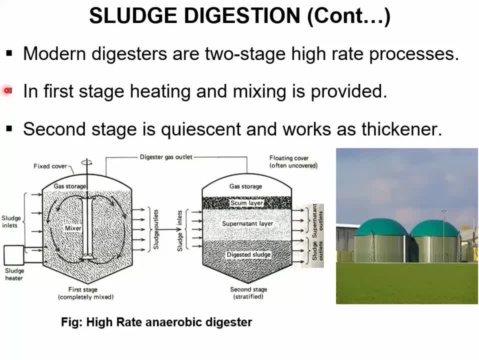 So this much is the Significance of the temperature. Therefore, In modern anaerobic digesters, They are both heated And mixed, And the temperature is normally maintained At close to 35 degree Celsius, And mixing is sufficient To completely intermix the contents. 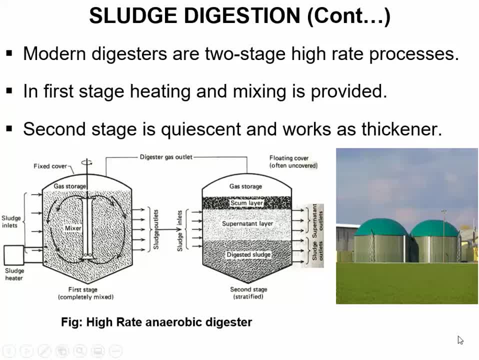 Once daily. The gases produced in anaerobic digestion Consists of 60 to 70 percent Methane by volume And the remaining Carbon dioxide And traces of Ammonia, nitrogen, hydrogen sulfide, etc. Because of the contaminants. 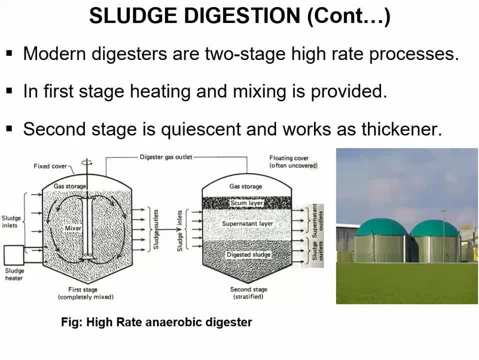 Particularly carbon dioxide And H2S. hydrogen sulfide, Methane is not a very good fuel. This mixture of gases Is not a very good fuel Because carbon dioxide Is not combustible And hydrogen sulfide Produces sulfuric acid. 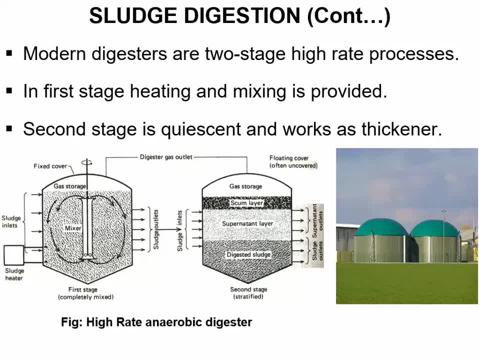 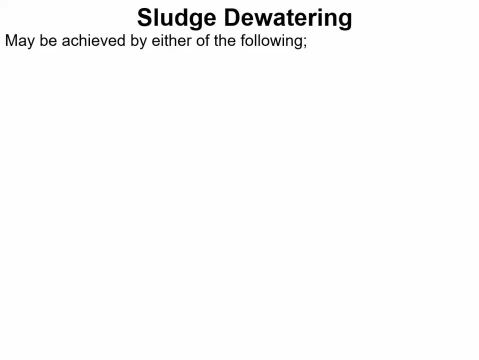 When it is burned. Therefore, It has to be removed From the gas, Separated from the methane, Before it can be used as a fuel gas. The next treatment unit is less dewatering. Dewatering processes May be usefully divided into: 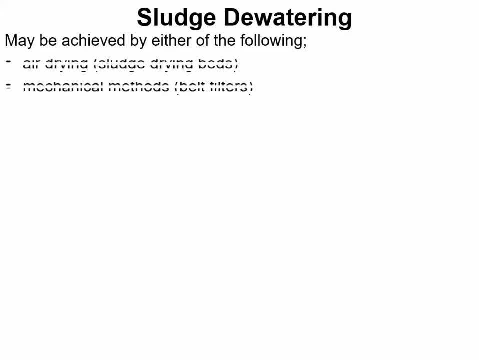 Air drying and mechanical methods. Air drying includes Those methods in which Moisture is removed by Evaporation and gravity, Or induced drainage, such as In the case of sand beds Or sludge drying beds, Whereas in mechanical methods, Such as bed filters. 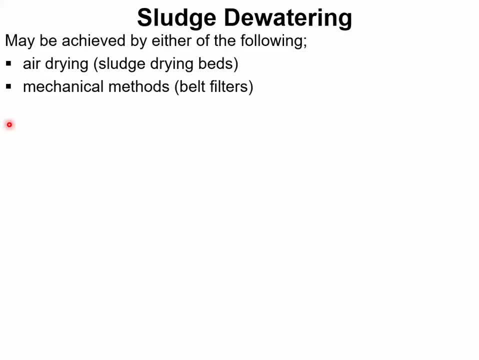 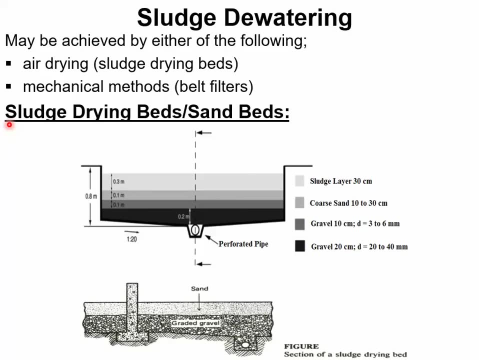 Mechanical techniques are used To separate water From the solids. Lets first talk about sludge drying beds, Or sand beds. Sand beds are the oldest Sludge dewatering technique And consists of around 100 to 300 mm. 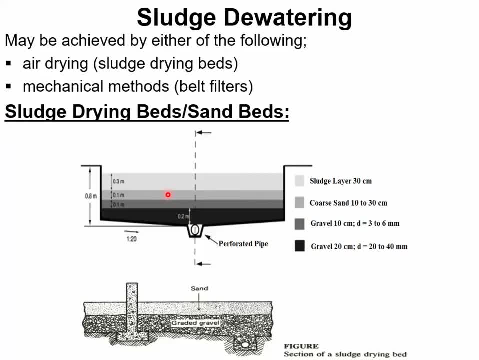 Layer of coarse sand, Underlain by Layers of graded gravel, Which is From 3 to 6 mm at the top And 40 mm At the bottom. This is the size of the gravels, The overall thickness of this gravel layer. 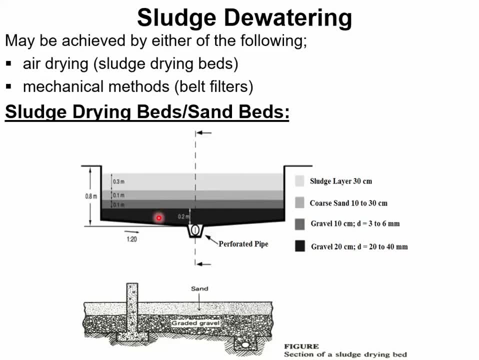 Is around 300 mm. The bottom of the sludge drying beds Is usually Natural, Graded to 100 or 150 mm. Drain tile From 6 to 9 meter centers, Side walls And partitions Between bed sections. 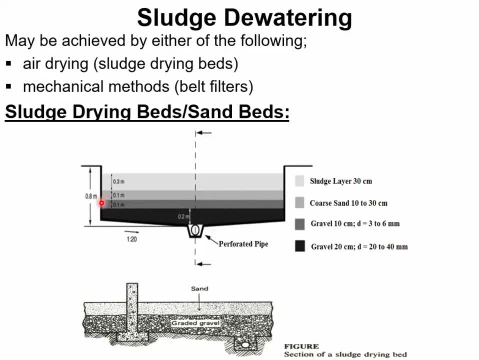 Are of concrete Or wooden planks And extend 300 to 400 mm Above the sand surface. Beds are operated By filling them With digestive sludge To a depth of around 200 to 300 mm, Dewatering occurs. 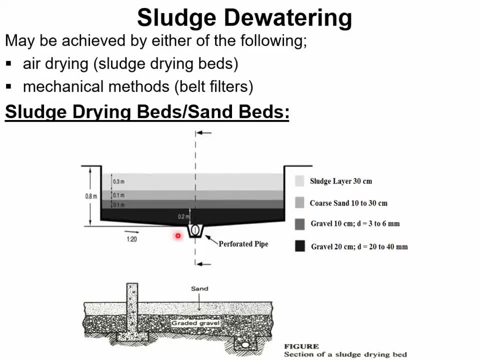 As a result of drainage, Water percolates down And evaporation, And is very much affected By the climate. In dry climates, Sludge will be Dewatered easily, Whereas in wet climates There would be some problem. 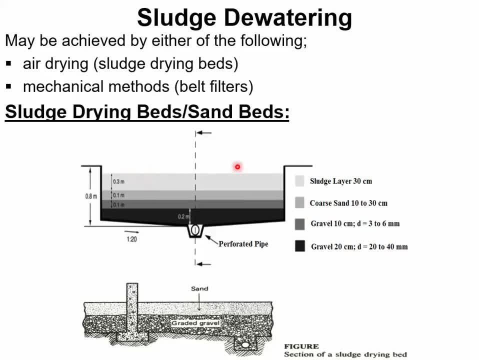 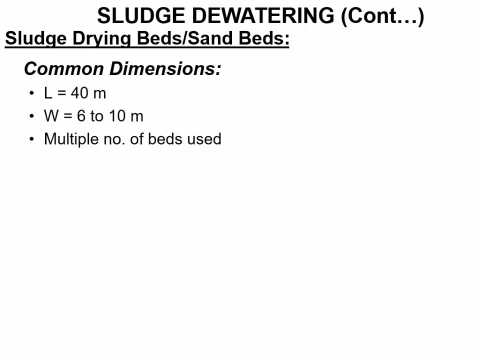 For dewatering. Therefore, covering the beds With glass or some other Has proven To be helpful In wet climates. The beds are 6 to 10 meter wide And up to 40 meter long, And at least two. 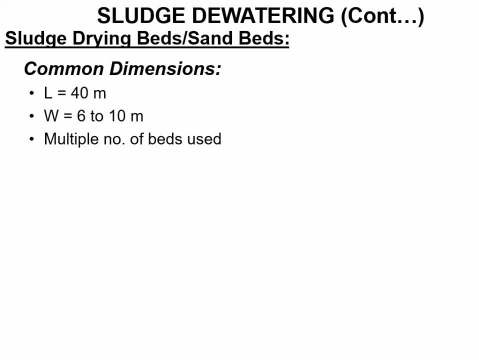 Beds are provided In even the smallest plants, Whereas in large to medium plants, Multiple number of beds Are required. Typical loading rates For digested sludges Range from 300 kg Of solids per square meter Of the sludge drying bed area. 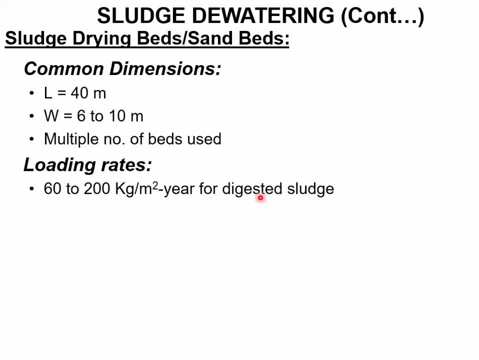 Per year For the digested sludge, Not for the raw sludge After digestion. This could be the loading rate To be applied for sludge drying beds. Drying takes from A few weeks to a few months, Depending upon the climate. 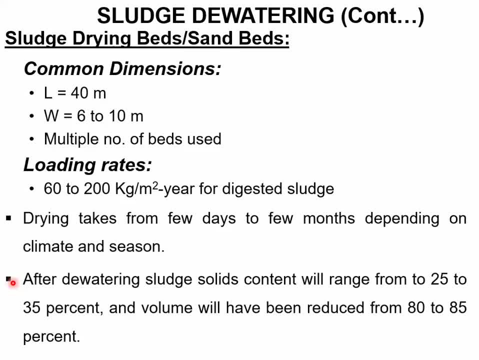 And the season, And after dewatering The sludge, solids contents Will range from 25 to 35 percent And volume Will have been reduced By 80 to 85 percent. The dried sludge Can be removed from the bed. 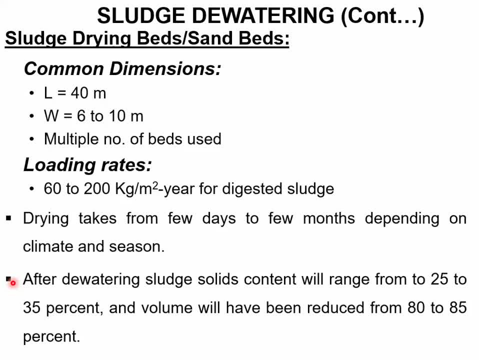 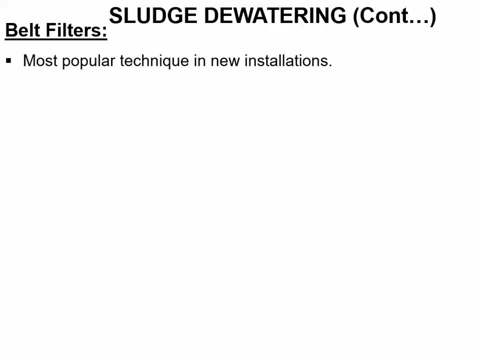 With light mechanical equipment Such as front end loaders. A small amount of sand Is lost in each drying cycle And the bed must be refilled periodically. Sludge drying beds Are one of the cheapest methods For dewatering of the sludge. 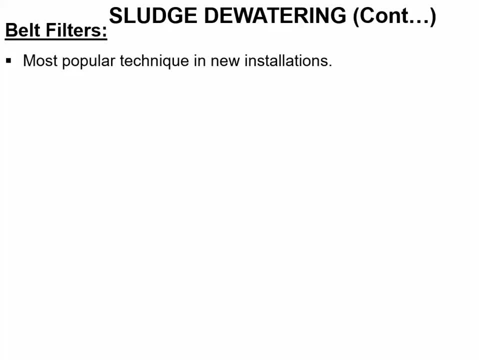 However, they require Very large land area Because the dewatering and drying process Is occurring naturally By air drying, By drainage and evaporation. The area required For sludge drying beds Can be estimated by the loading rates Given on the previous slide. 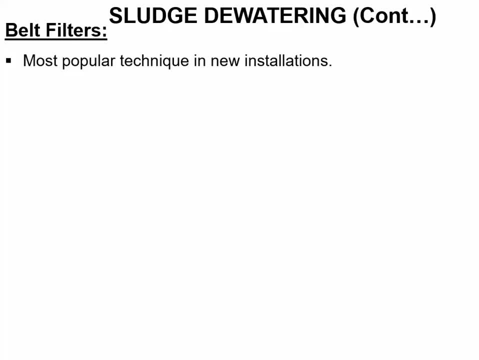 So for such applications, Where land area Availability Up to the requirement Of the sludge drying beds, Where land spaces are limited, For example in industries, The mechanical dewatering processes Are used there. Mechanical dewatering processes. 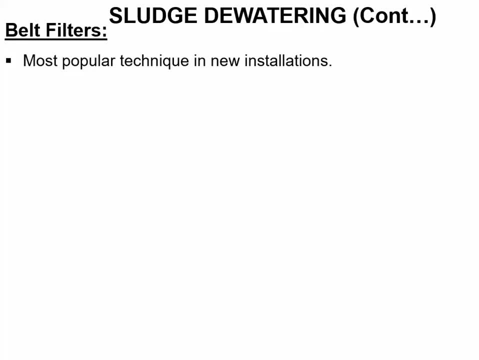 Include bed filters, Pressure filters, Vacuum filters And a number of other similar devices. Out of all these, Bed filters have become The most popular sludge dewatering device In new installations Because the capital cost And operating costs 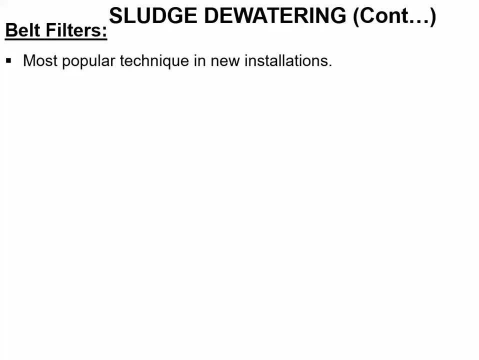 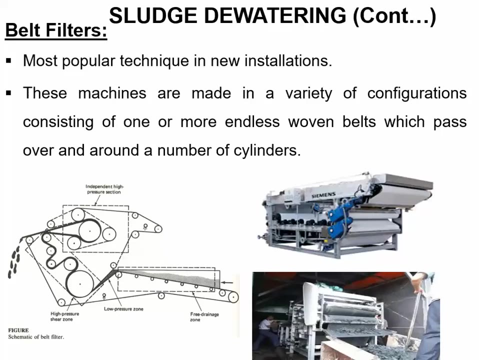 Are generally less than Other mechanical techniques, And they also produce a sludge Which can be handled as a solid. These machines Are made in a variety Of configurations Consisting of one or more Endless woven beds Which pass over and around. 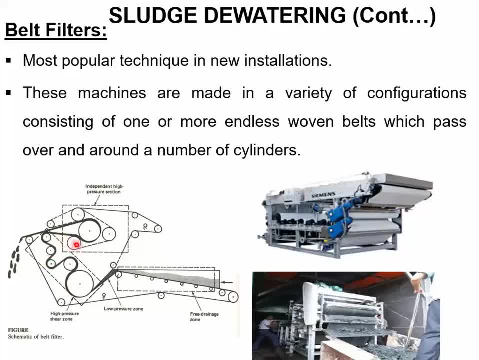 A number of Standards. So in most designs The chemically conditioned sludge Is fed To an open bed surface On which the gravity drainage occurs. As the bed moves forward, The gravity drainage would occur At the end of the gravity drainage. 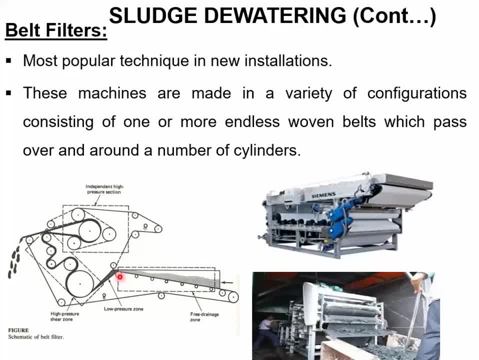 Section. This section, Provided the sludge Has been properly conditioned, The solids contained here Should be 10% or more. At this, moisture content Of 90% or lesser, It behaves as solid And can be subjected To pressure, shear and vacuum. 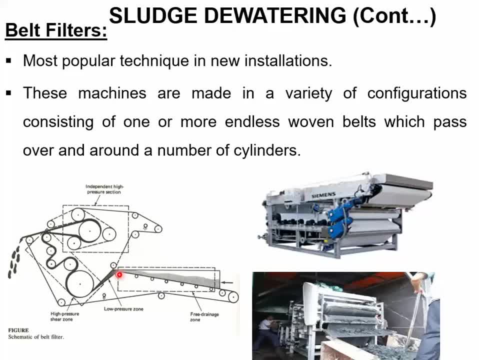 In the subsequent subsections Of this belt filter. A second belt Is then brought Gradually, brought down Towards the moving sludge At the end of this gravity zone And gradually applies pressure To the solids To let out additional moisture. 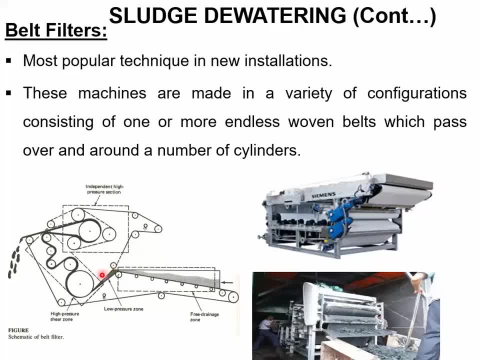 As the paired belt Move around These rollers, Their speed relative to each other varies And the sludge mass is sheared, Aiding in release Of the free water. The pressure gradually increases Through the machine And, in some designs, 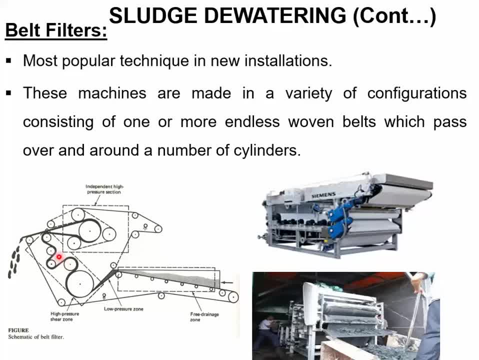 A partial vacuum is also applied. The belts then separate at the end And the sludge cake Is dislodged By scrapping the belt Or by passing it around A very small radius roller. So this Product can be expected. 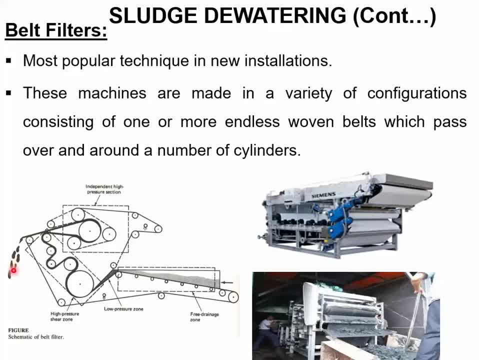 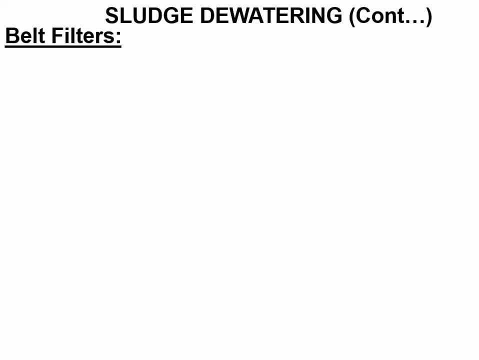 To have solids content In the range of 12 to around 40%, Whereas 20% is the typical value Of the solids content In this sludge obtained. As I mentioned On the previous slide, The addition sludge is applied. 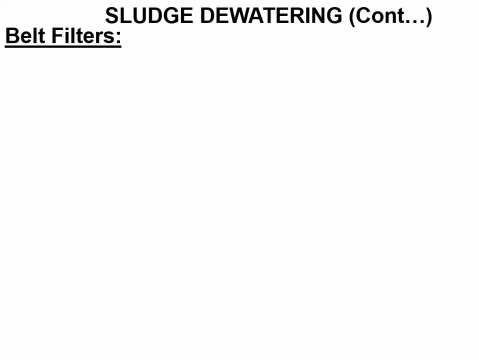 On the belt filters. So why Chemical conditioning is required? Because it is not easy To separate water From the solids In natural processes Such as sludge drying beds. Since long retention times are provided, Therefore, conditioning is not required. 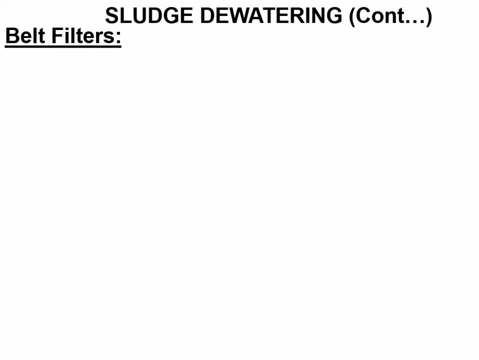 Digested sludge can be applied Directly to sludge drying beds, Whereas for mechanical Dewatering processes In the belt filters, Sludge has to be first chemically conditioned So that Dewatering can be enhanced. So chemical additives. 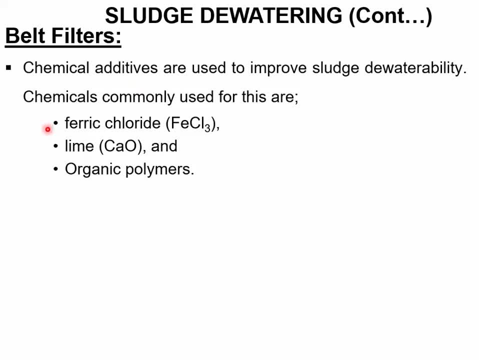 Which are used Commonly for this purpose To enhance the sludge dewaterability, Include ferric chloride, Lime And organic polymers. The product from the belt filter I have already mentioned that Can be expected to have Drain from 12 to 40 percent. 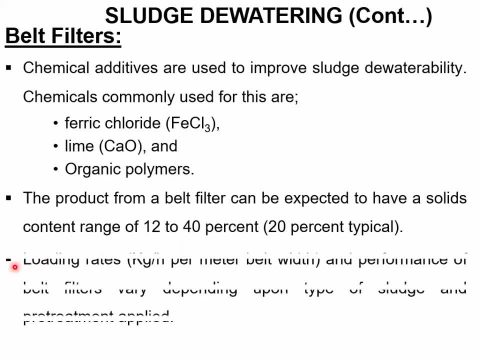 With 20 percent Being the typical value. Loading rates For the belt filters Are in the units of kilograms Per hour per meter Of the bed width. These loading rates And the performance of the belt filters Vary depending upon the type of the sludge. 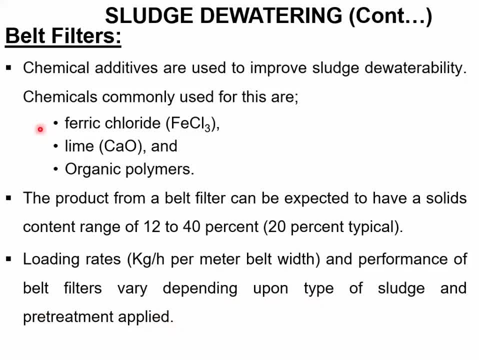 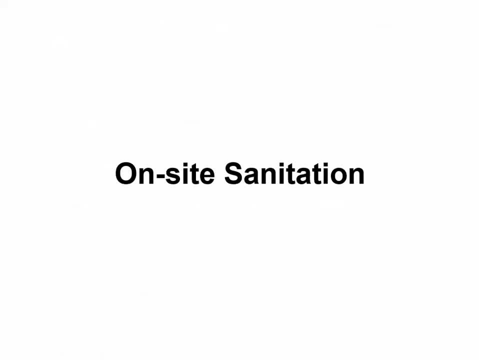 And the pre-treatment applied With the help of these chemicals. So next We are going to discuss A very brief topic of on-site sanitation. On-site sanitation means The sewerage facility required At construction sites Where proper sewerage system. 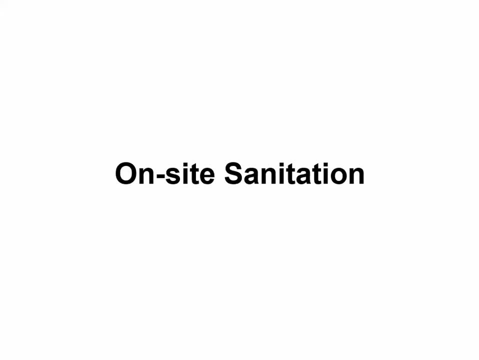 Is not available, And at such sites Or such communities Where The proper sewerage system Is not installed And is not economical to install. Therefore, For each house, The sewerage system can be used To dispose of its waste water. 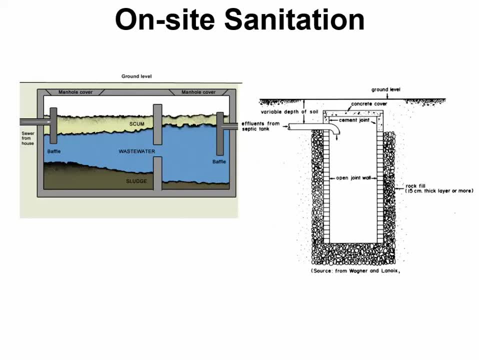 So typical On-site sanitation Is employed using the first A septic tank, And then effluent from the septic tank Is disposed of through a soak away Or soakage pit Or a drain feed. Let's discuss about these two units. 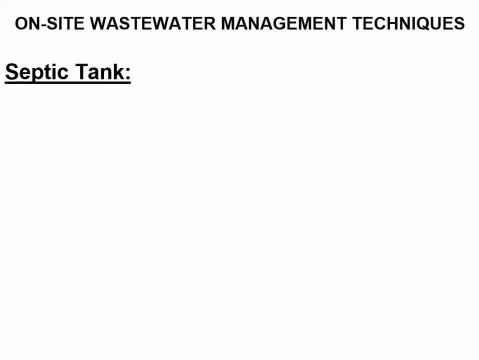 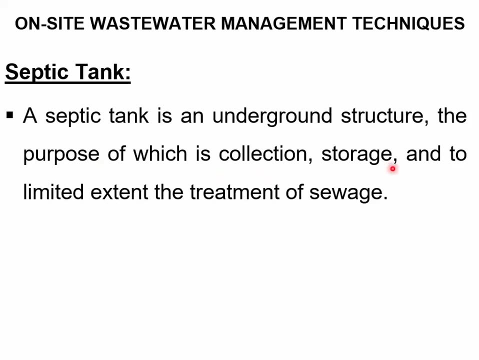 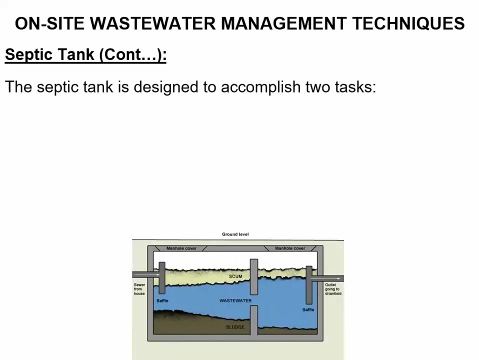 Individually. So first About the septic tank. It is an underground structure. The purpose of it is collection, Storage and to some extent The treatment of sewage, So it also does Partial treatment of sewage. So the septic tank is designed. 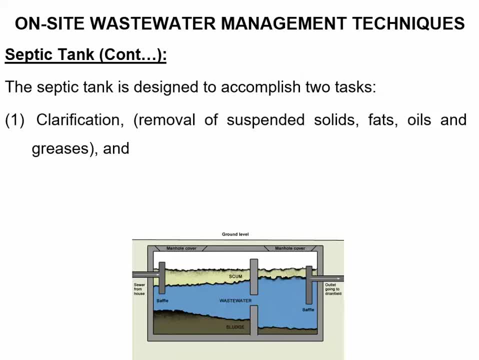 To accomplish two tasks: First the clarification, That is, the removal of suspended solids Primarily, And then other things Such as fats, oils and gases, And the treatment, Which is partial decomposition Or partial oxidation Of the settled organic matter. 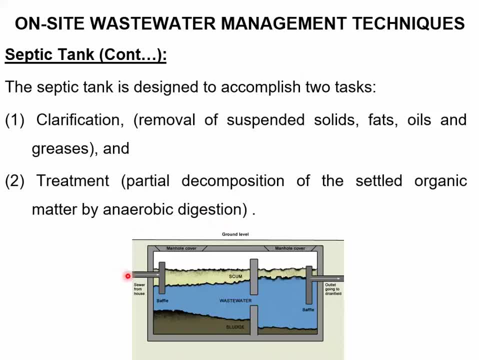 By anaerobic digestion. So what happens is that Waste water from a house Comes to a two compartment Or three compartment septic tank. The suspended solids, Which are Organic suspended solids Of domestic waste water, They settle down at the bottom of the first compartment. 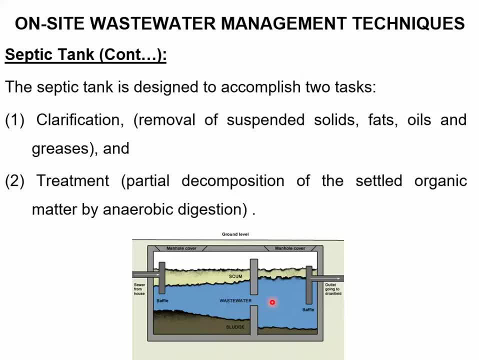 And the rest of the Suspended solids which are remaining. They can also settle at this Bottom of second compartment. So these settled suspended solids Then Undergrow anaerobic decomposition By bacteria, So organic matter is oxidized into. 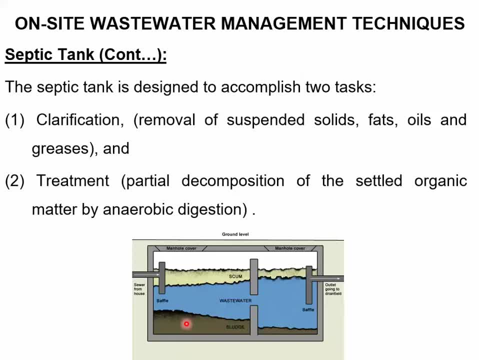 And products Of typical anaerobic decomposition, Such as H2S gas, Methane gas, Carbon dioxide, etc. The lighter particles, Such as oil and grease particles. They accumulate At the top surface of the septic tank And clearer water. 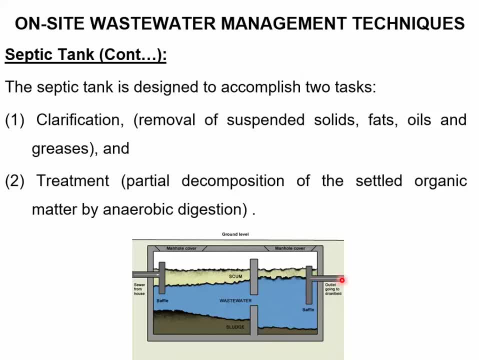 Goes to the second compartment And from there to the outlet, To the drain field Or soakage pit. So we are discussing The septic tank As part of wastewater Disposal. So prior to disposal through a soakage pit. 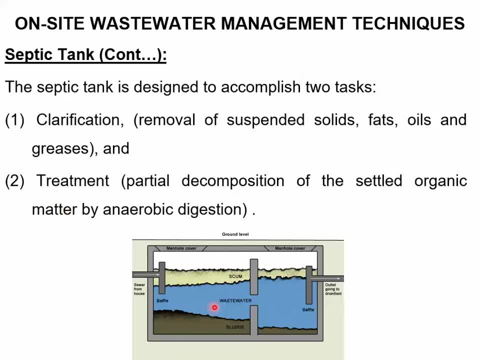 The wastewater is settled, Is clarified and partially treated So that relatively clear water Is disposed of into the soil, Using the soak away. However, As I mentioned while talking about The sewer system design, That septic tanks are also Applied nowadays in urban areas. 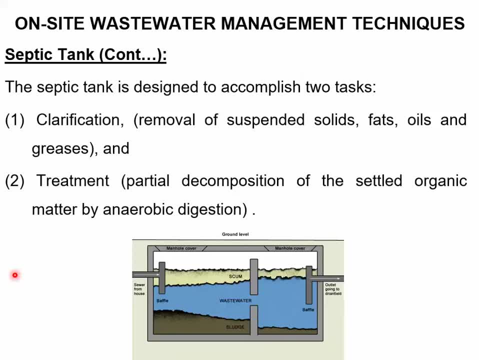 As part of the bylaws, And every house septic tank Is mandatory To achieve the clarification of the Sewage prior to its discharge Into sewer system. The objective of that is That the suspended solids Which have settled here 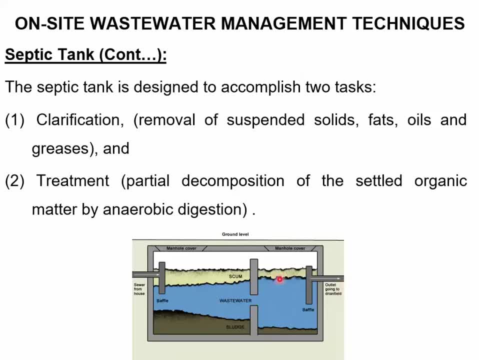 Should not go to the sewer system, Such as: And. similarly, the grease And oil should not go to the sewer system. So the problems, The operational problems Of the sewer system Are avoided or eliminated Or reduced to some extent. The partially treated effluent. 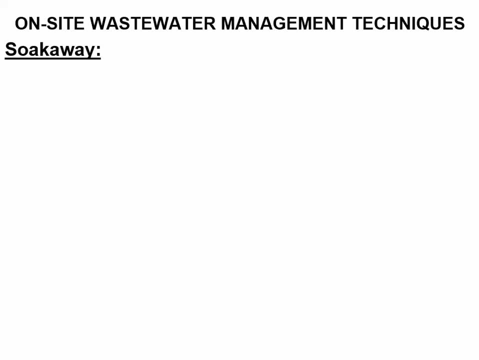 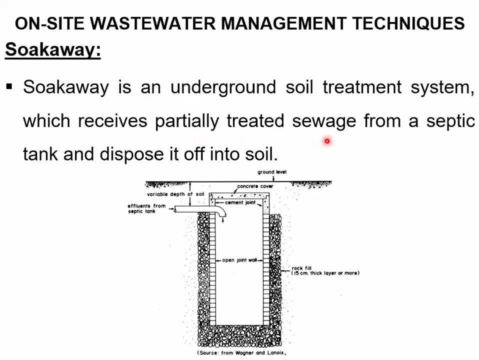 Of the septic tank Is then further disposed of Into the soil With the help of a soak away, A drain field, Or it is also called as soakage pit. Soak away is an underground Soil treatment system Which receives partially treated sewage. 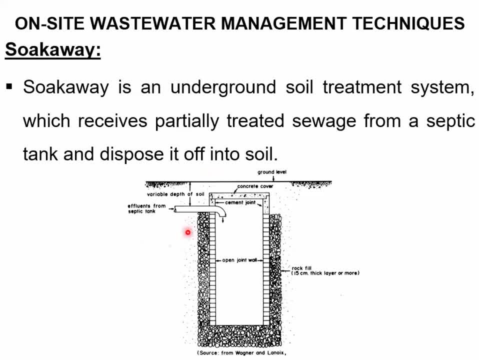 From a septic tank And dispose it off into the soil. So this is Effluent coming from the septic tank. It is disposed off into this Soakage pit. This pit is just like a brick Manhole, you can say. 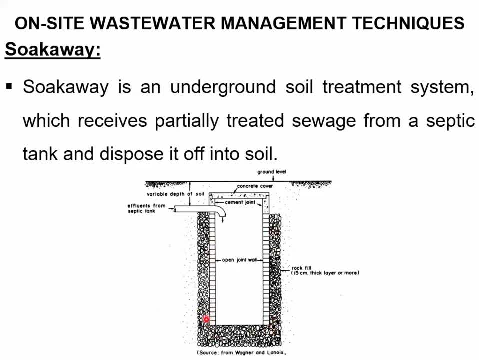 The walls are brick And it is rock filled Around. Around 15 cm Thick layer, or More thickness Can also be provided. This is the rock filling around This soakage pit. So base water Which is partially treated. 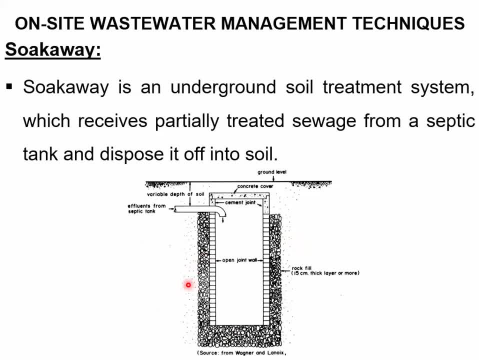 Would percolate into the soil Through its bottom And through its sides And will get the treatment Through the soil filter, The soil. Since it is a natural filter, It can remove conventional pollutants- Almost all of the conventional pollutants.